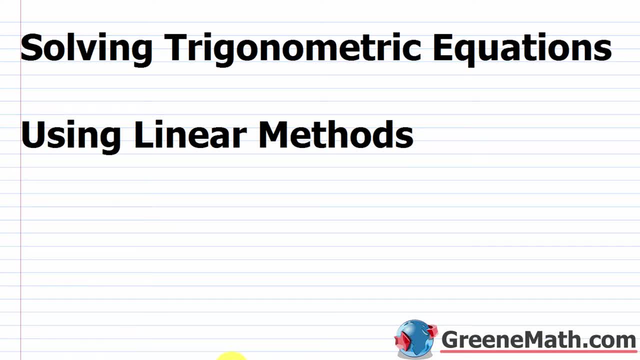 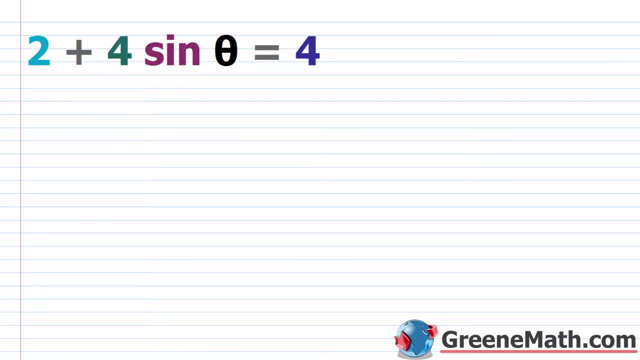 In this lesson, we want to talk about solving trigonometric equations using linear methods. All right, so let's start off with the easiest possible scenario. We're going to solve some trigonometric equations, again, with these linear methods. Let's say you had something like 2 plus 4 times the sine of theta is equal to 4. So what we're trying to do here, we're trying to find values of theta, okay, that I could plug in here and make the equation true. Now before I go through this, let's just look at something from basic algebra, so we'll remember this. If I had something like 2 plus 4x is equal to 4, how would I solve this? Well, I'm trying to find values for x that make the equation true, right? So I would first try to isolate x, so I would subtract 2 away from each side of the equation, and so this is going to cancel. I would say 4x is equal to 2, divide both sides by 4, and I get that x is equal to 1 half, okay? So I plug a 1 half in there, and basically you have what? You have 2 plus, basically 4 times a half is 2, so 2 plus 2 gives me 4, so that is the correct solution. With this guy, it's not as straightforward, it's not as easy, because remember you're plugging in an angle measure there, sine of that guy would give you a number, okay? So you're looking for sine of some value, I can already tell you that this needs to be a half for this to be true. So where is sine of theta equal to a half, okay? That's what you're going to be looking for. 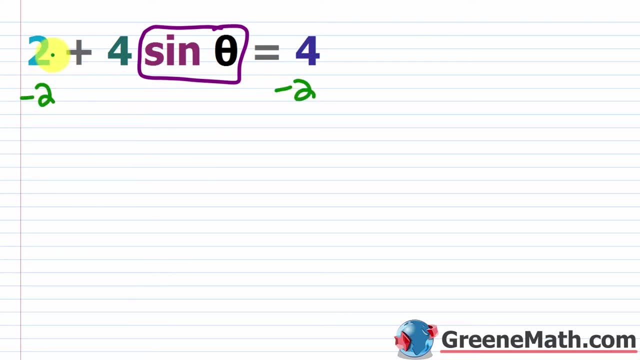 But to solve this fully, let me subtract 2 away from each side of the equation, 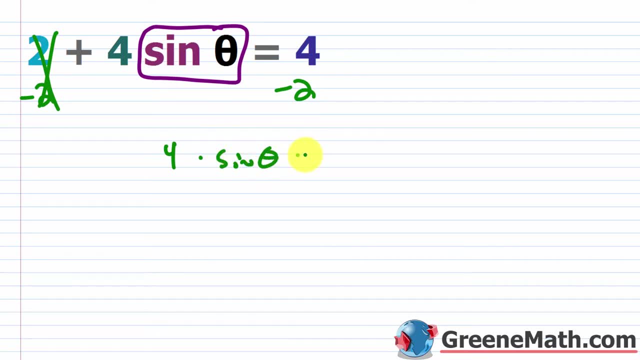 this cancels, we get 4 times the sine of theta is equal to 2, we divide both sides by 4, and basically we're going to get that the sine of theta, again, is equal to a half, okay? So from 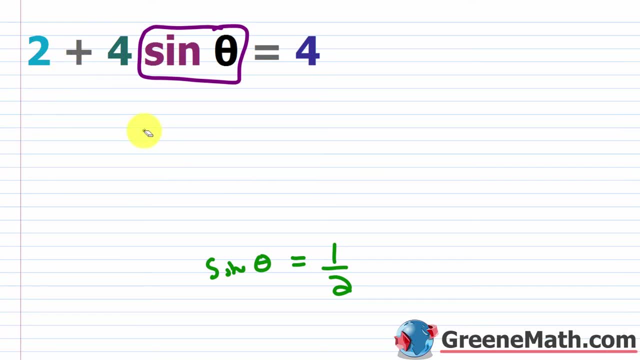 this guy right here, this is where you need to basically do a little bit of detective work, 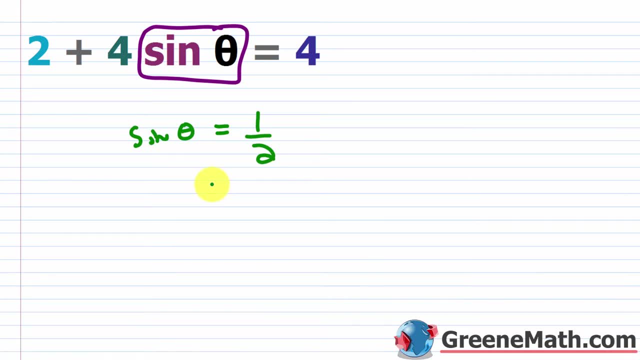 okay? There are so many ways to solve this, it's not even funny. You might want to use a calculator and use your inverse sine function, you might want to use the unit circle, there's a lot of 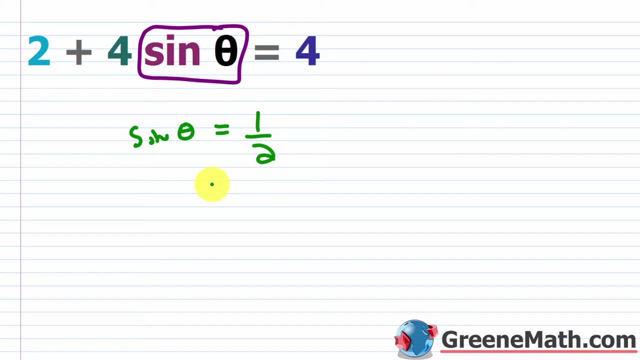 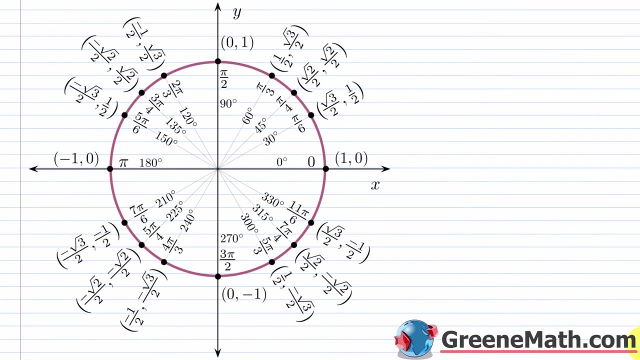 different things that you could do. You could use the special triangles that you remember, all kinds of ways. So let me talk about two ways that you can solve this. First, let's think about the unit circle approach. So if you are lucky and you get an easier problem where basically you can 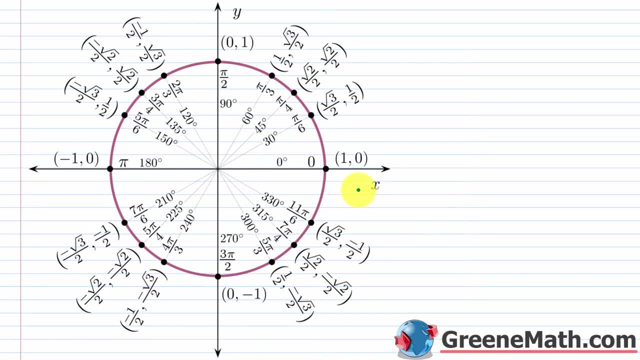 find this from the unit circle, you can go to the unit circle, if I'm looking for sine of theta is equal to a half, well you can look for the y-coordinate and find out where it's a half, okay? So for 30 degrees or pi over 6 in terms of radians, the y-coordinate is a half, right? 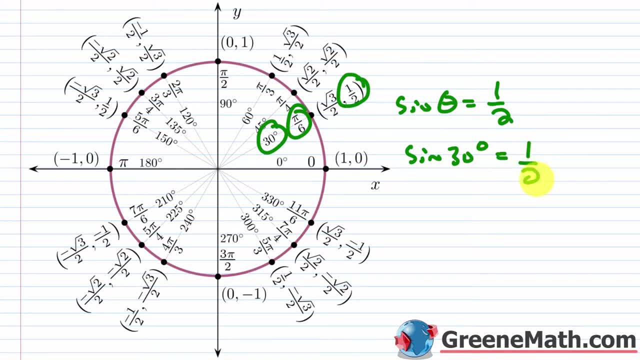 So that tells me that sine of 30 degrees is equal to a half. Then also, I know that sine is positive in quadrant two. 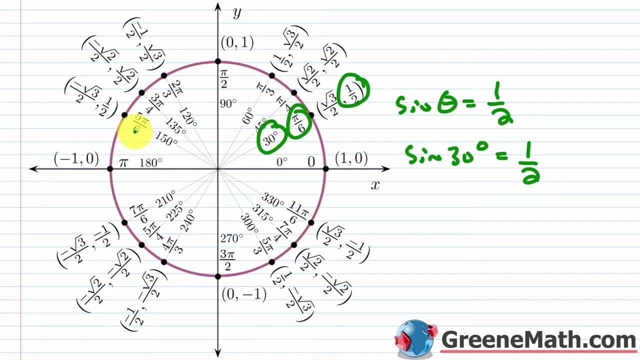 So remember, when we think about reference angles, if the reference angle is 30 degrees, then sine of that guy is also going to be a half, right? So where would I have a reference angle of 30 degrees? Well, with 150 degrees, right? Because 180 degrees minus 150 degrees, the reference angle would be 30 degrees. So sine of 150 degrees, sine of 150 degrees, and I'm messing up my writing there. So sine of 150 degrees would also be a half, right? And you can see that here. 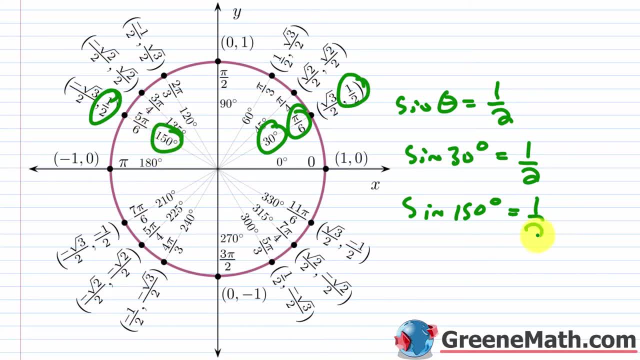 This is a half, this is 150 degrees, or 5 pi over 6 if you're talking about radians. 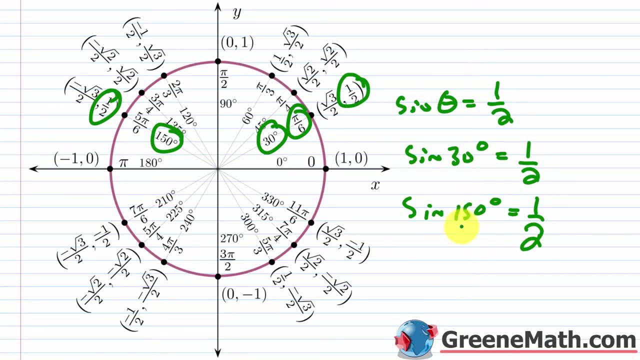 Now, when you talk about solutions over the interval, from if you think about zero to 360 degrees, your solutions would be 30 degrees and 150 degrees. But when you think about a general solution, remember, when you think about sine and cosine, the period is 360 degrees or 2 pi, okay? So that means if I started here and I rotated around 360 degrees, well, instead of 30 degrees, now I'd have 390 degrees, and sine of 390 degrees would also be a half, okay? 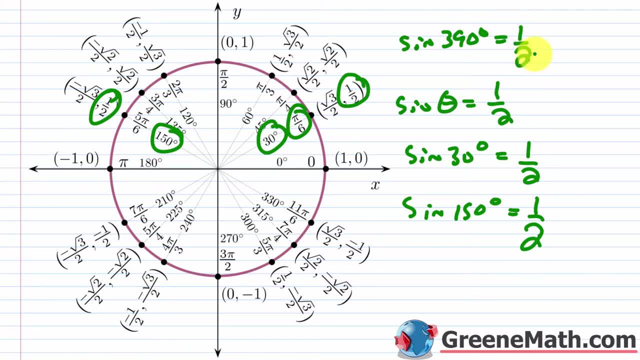 If I added 360 degrees again, then sine of, in that case, 750 degrees would also be a half, you know, so on and so forth. Same thing with 150 degrees. 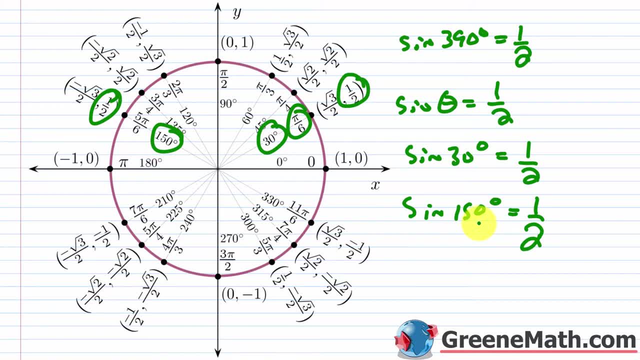 If I add 360 degrees, I'm going to be at 510 degrees, sine of that guy would be a half as well, okay? 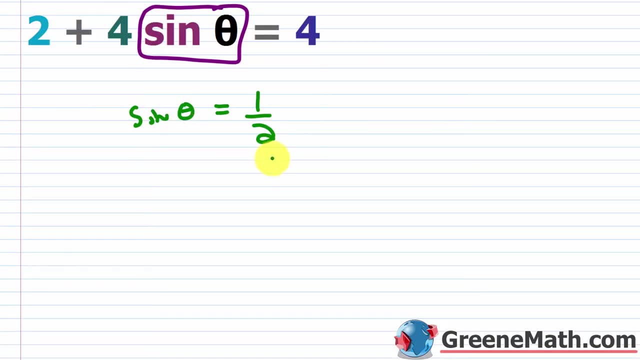 So let's take that information and come back. And give a solution, okay? 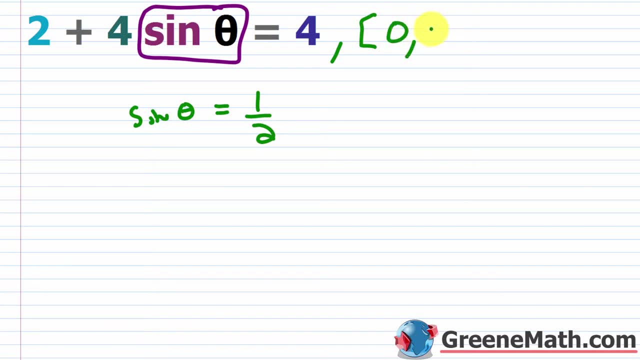 So first, let's pretend we're restricting the domain, so zero to 360 degrees, or again, you might see this in terms of radians, so you might see zero to 2 pi in terms of radians. 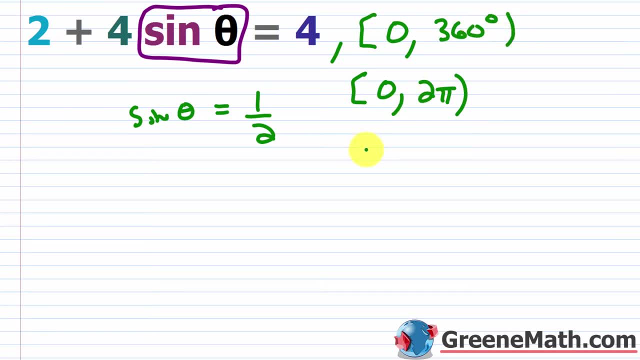 Whatever you get, you want to match that in terms of your answer, okay? So if you get degrees, put degrees. If you get radians, put radians, okay? So in this case, I'll just do both. 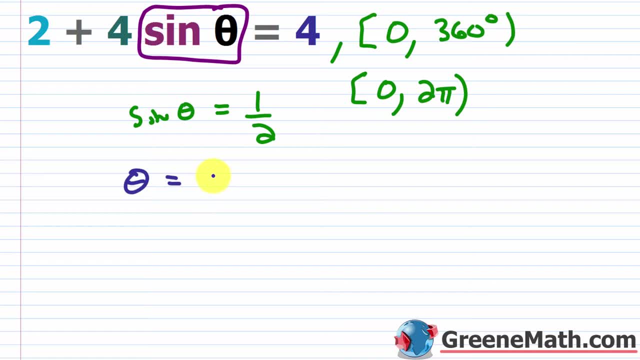 So in this particular case, I'll say that theta is equal to, we had 30 degrees and then also 150 degrees. And again, you know the reference. The reference angle for both of those is going to be 30 degrees. And then if we look at, in terms of radians, we could say theta is equal to pi over 6, this is 30 degrees in terms of radians, and then 5 pi over 6, this is 150 degrees in terms of radians. Now, this is the solution for the restricted domain. 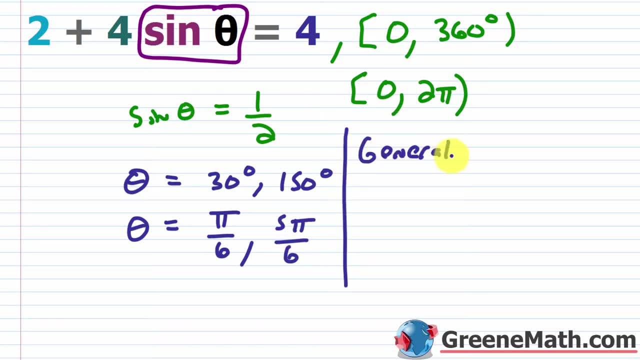 If you want a general solution, so let me put the general solution, okay? So this is going to keep working as we either rotate clockwise or counterclockwise. So remember, if you go 300 degrees, you're going to get a general solution. If you go 360 degrees, it doesn't matter which direction. If you go negative direction, so you're going clockwise, or you go the positive direction, so you're going counterclockwise, you're going to keep getting these guys, okay? 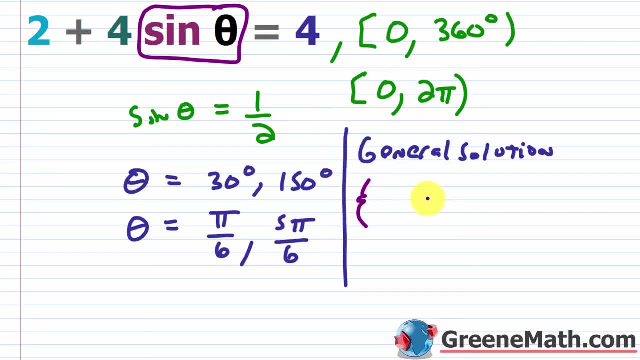 So I'm going to start with, let me make some set braces here, okay? This is typically how you'll see it. I'm going to take this solution. You could do it degrees or you could do it radians. I'll do both. 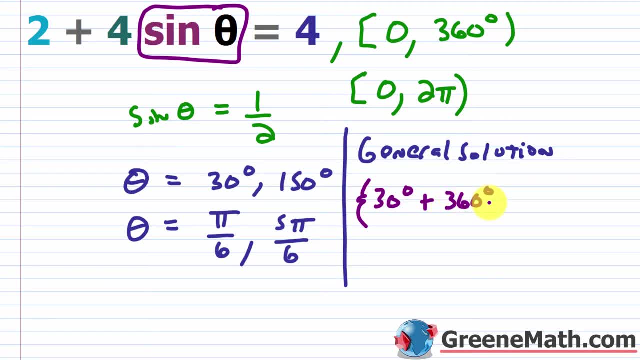 So 30 degrees plus the 360 degrees, okay? When you go around, again, you're going to get that same value and then times n, where n is just any integer, okay? 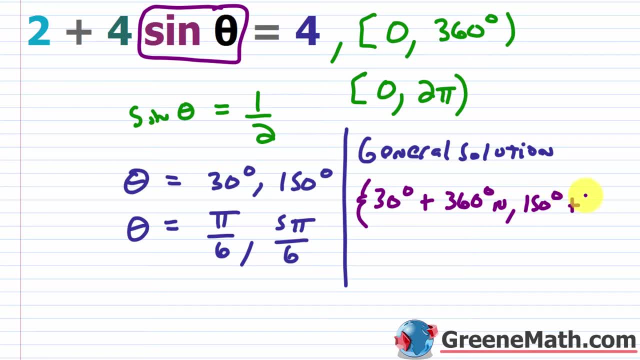 And then I'm going to do 150 degrees. And then plus this 360 degrees. Let me slide all of this down because it's not going to fit. So let me move this down. And let me put this comma back where it should be, right there. 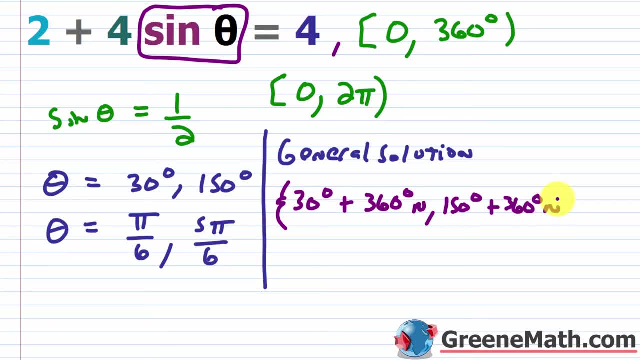 Okay, so this, I'll close my set braces and I forgot my n. So let me put the n there, okay? 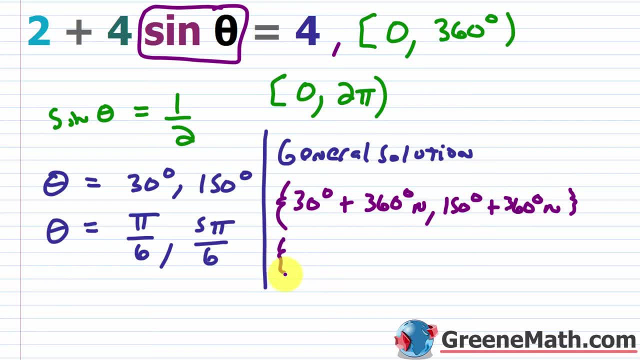 So that's your general solution in terms of degrees. With radians, you would say pi over 6 plus, remember, 360 degrees is just 2pi, okay? 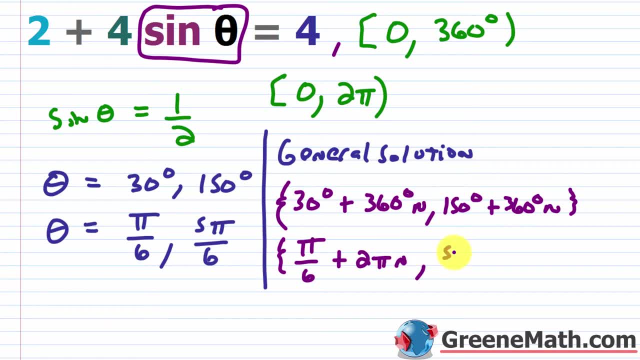 So I'm going to put 2pi n, and then I'll do 5pi over 6 plus 2pi. 2pi n, okay? So there's your general solution. 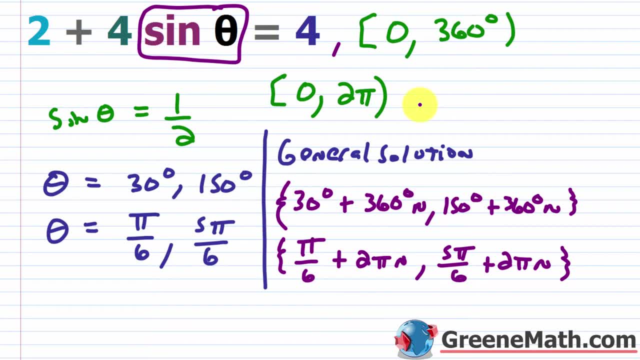 There's your solution for having this domain restriction, okay? Where basically you're between 0 and 2pi. Or if you think about this in terms of degrees, 0 and 360 degrees. 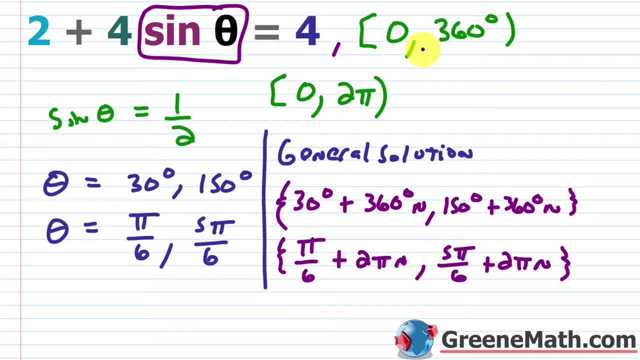 Now, let's talk about another way that you could have gotten this answer. In a lot of cases, especially harder cases, you're not going to be able to use the unit circle, okay? 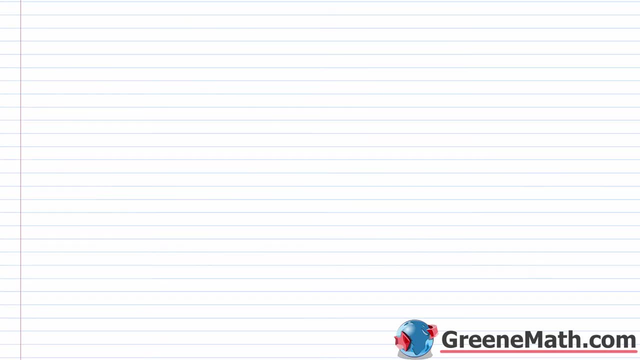 So what you want to do is use your inverse sine function. So let me use a fresh sheet here. Let's say I looked on my calculator and I did inverse sine. 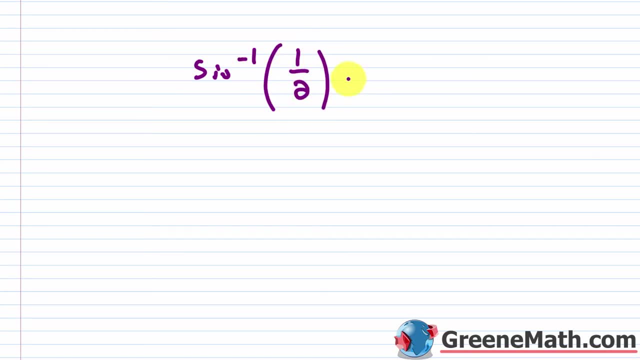 Of, in this particular case, we were looking at a half, okay? 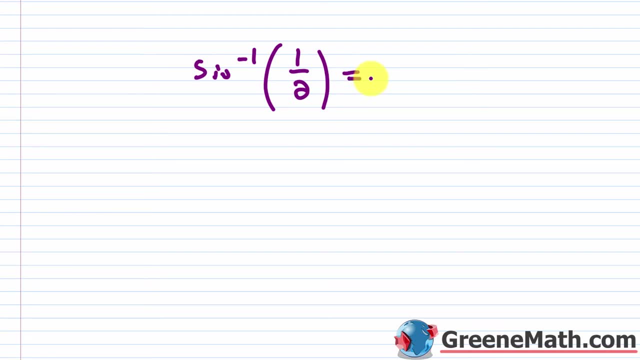 So you punch this into your calculator, and we already know you're only going to get one value, right? You're just going to get 30 degrees, okay? 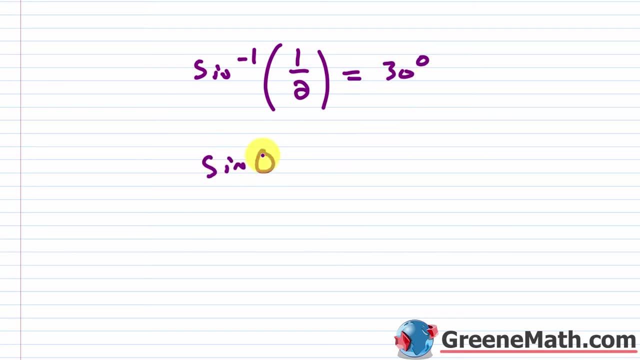 But again, if I think about sine of theta is equal to one half, there's an infinite number of angle measures there that's going to be true for this. And if I have one of them, then I can find all of them. Again, because where is sine positive? It's positive in quadrants one and two, okay? So I have the answer from quadrant. One, I have my answer from quadrant one. It's going to be 30 degrees. And again, it repeats. 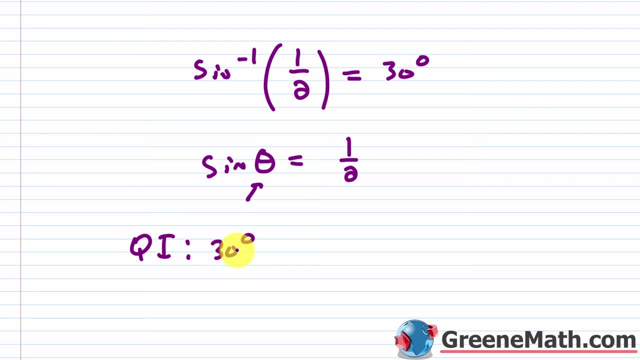 So 360 degrees in either direction. So if I go plus 360 degrees, or if I go minus 360 degrees, I'm going to, again, run into another solution. 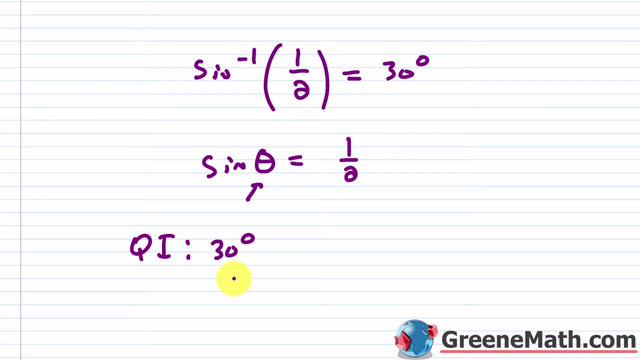 But in quadrant two, I just need an angle where the reference angle is 30 degrees, okay? So again, that's going to be found by taking 180 degrees. So I would take 180 degrees, okay? Minus 30 degrees. 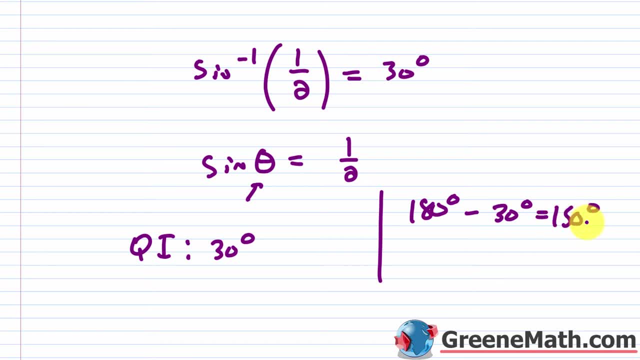 And that gives me 150 degrees, okay? So this is the angle I'm looking for. So in quadrant. 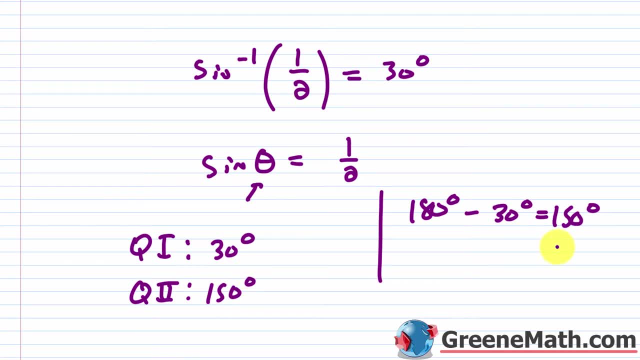 Two, I get 150 degrees. So that's another way that you could solve this. 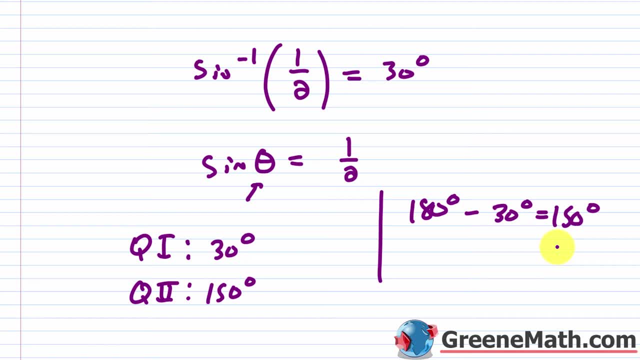 You could also use special triangles if you wanted to, okay? So there's a lot of different ways to think about this guy. Okay, let's look at another example. So we have the cosine of theta now instead of the sine of theta. 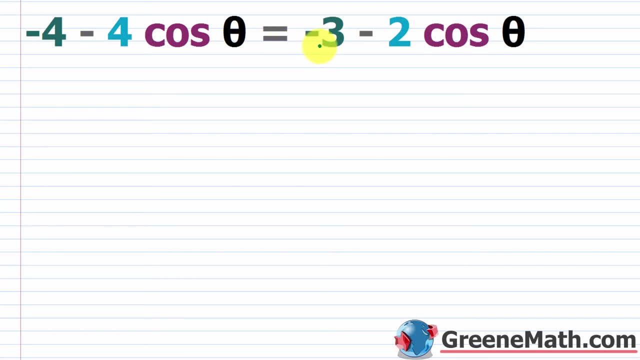 So we have negative four minus four times the cosine of theta is equal to negative three minus two times the cosine of theta. 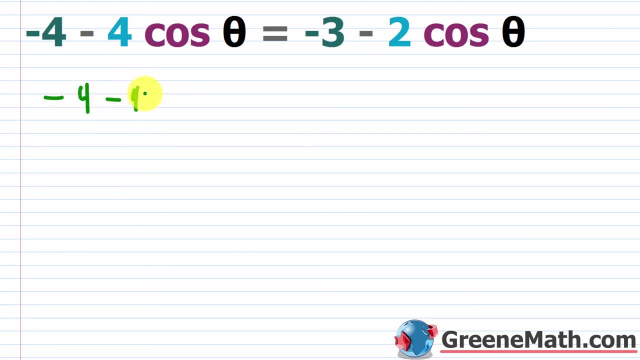 And again, if you're working with this, let's say you had something like negative four minus four x is equal to negative three minus two x, well, I'd want to get all the terms that x on one side, all the numbers on the other. Same thing here. I'm going to get all the terms with cosine of theta involved on one side, all the numbers to the other. 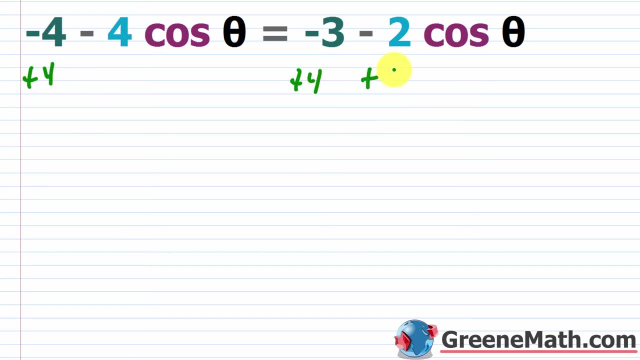 So let me add four to both sides, okay? And let me add two cosine theta to both sides, okay? And basically, we see that over here, this is going to cancel. 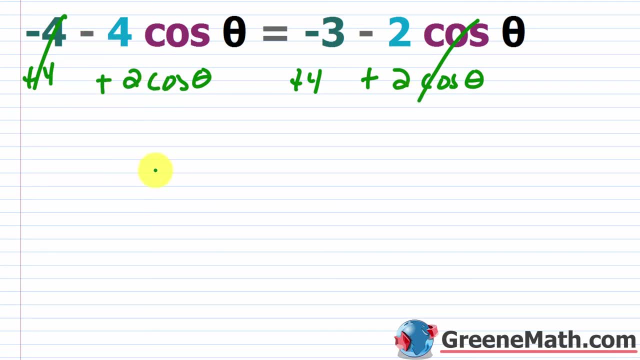 Over here, this is going to cancel. So I have negative four plus two, which is negative two, times the cosine of theta is equal to negative three plus four, which is one, okay? 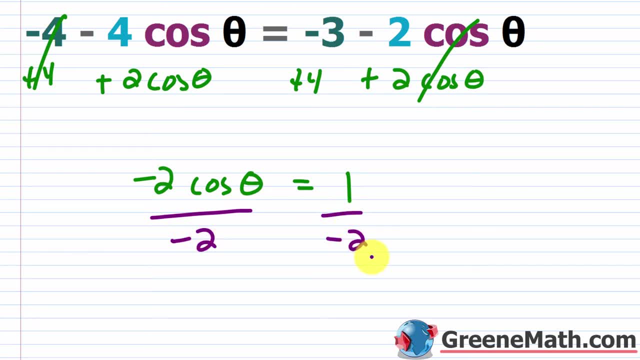 To isolate this guy, I'm going to divide both sides by negative two, and I'm basically going to find that the cosine of theta is equal to negative one half. 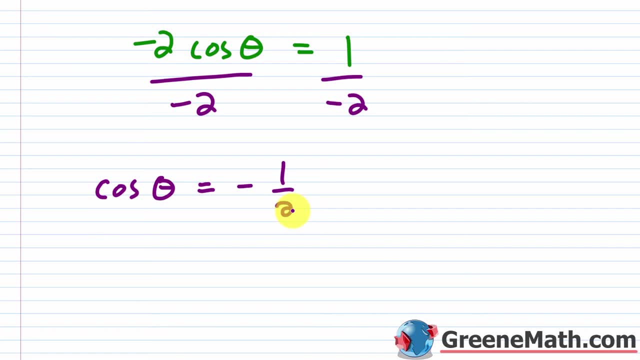 Again, another easy problem where you can get this from the unit circle, but let's go ahead and use our inverse cosine function. So let's go cosine inverse of negative one half, and let's do a little bit of detective work. 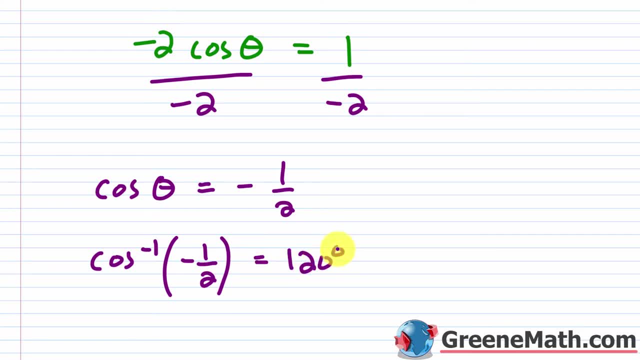 If you punch that in on a calculator, you're going to get 120 in terms of degrees, okay? 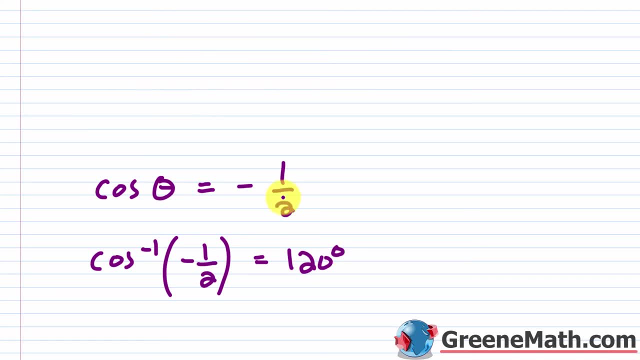 So let me erase this so I can drag this up. We'll have a little bit of room. 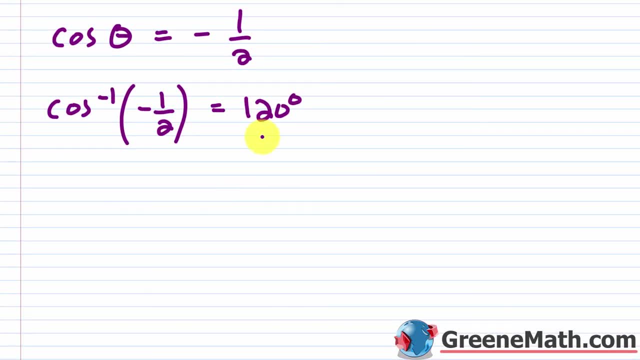 Okay, let me bring this up. And let's think about this. 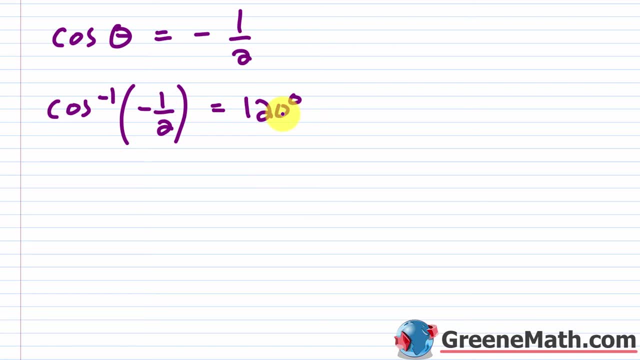 So I have 120 degrees there, okay? So in terms of the reference angle for that, remember, if you're in quadrant two, the reference angle is 180 degrees minus your angle, which is 120 degrees. So this is going to be 60 degrees. 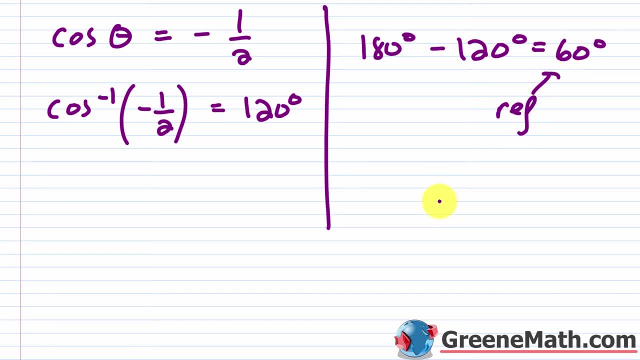 So this is my reference angle, okay? So what I want to do now, again, because this is negative here, cosine is negative in quadrant two. 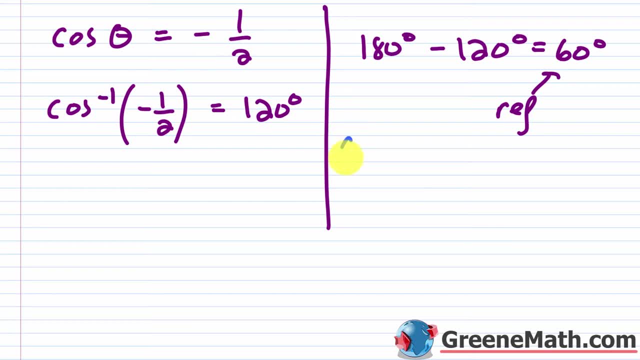 So I have my quadrant two solution. My quadrant two solution is 120 degrees. 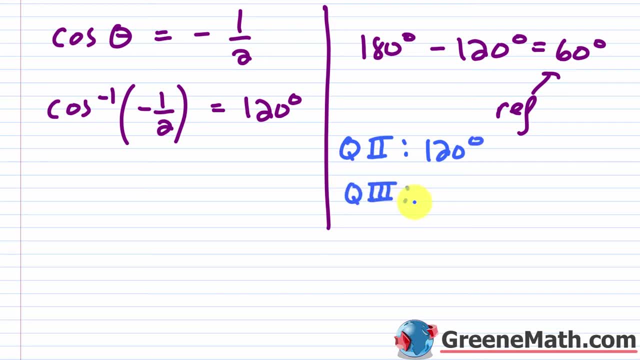 For my quadrant three solution, I want to think about an angle in quadrant three, okay, that has a reference angle of 60 degrees. How do I find that? Well, in quadrant three, I would want to take 180 degrees, and I would want to add to that 60 degrees, which is my reference angle, okay, which would give me 240 degrees, okay? This is 240 degrees. 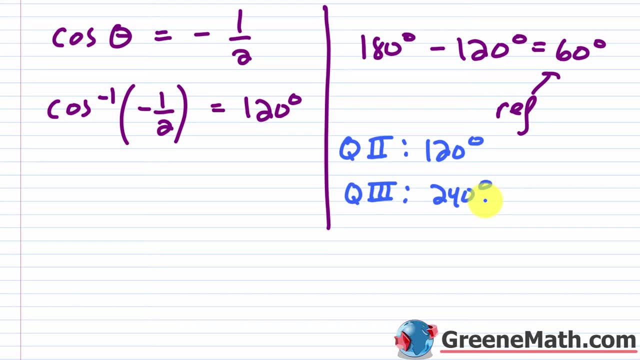 And the reason that works is, again, if I had a 240-degree angle, and I said, hey, what's the reference angle? 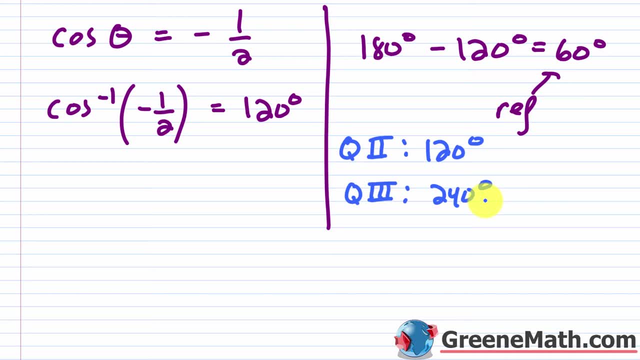 You would subtract 180 degrees to get 60 degrees, okay? So this is my answer in quadrant two. This is my answer in quadrant three, okay? 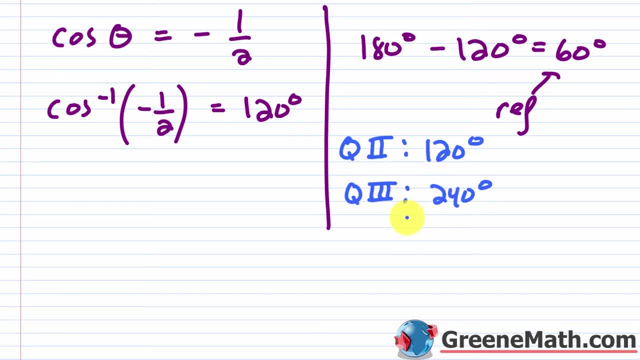 Now again, if you wanted a general solution, so let's pretend that first you got a domain restriction from zero to 360 degrees, like this, and then also in terms of radians, we have zero to two pi, okay, like this. So for the degrees... 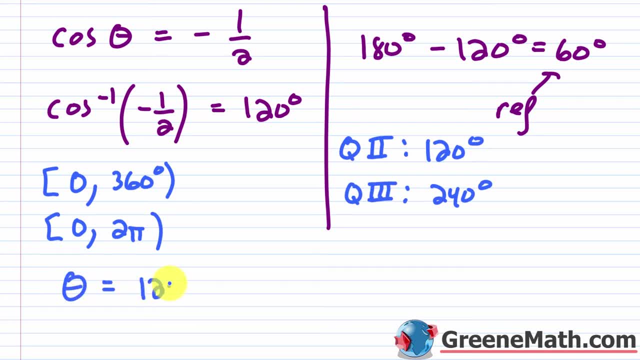 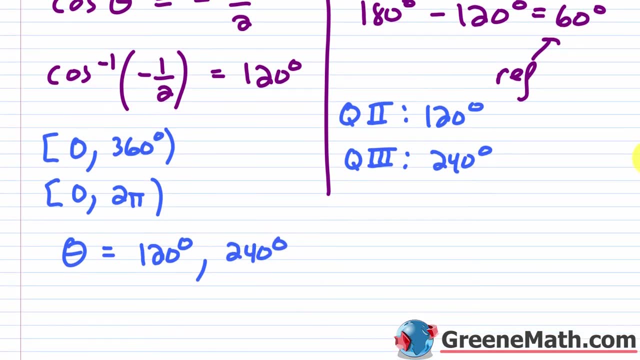 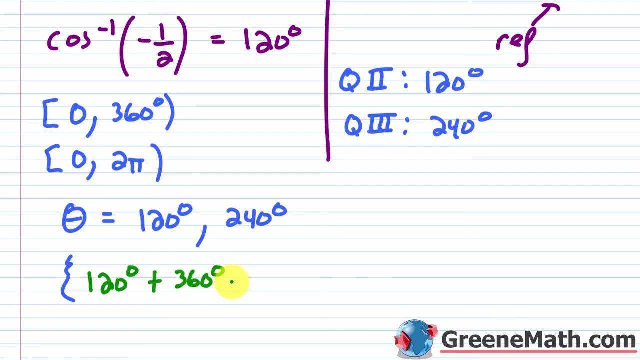 For the degrees, you would just put that theta is equal to 120 degrees, okay, and then 240 degrees. And then for your general solution, again, all you have to do in this particular case is, let's use some set braces here, and we'll say 120 degrees plus 360 degrees times n, 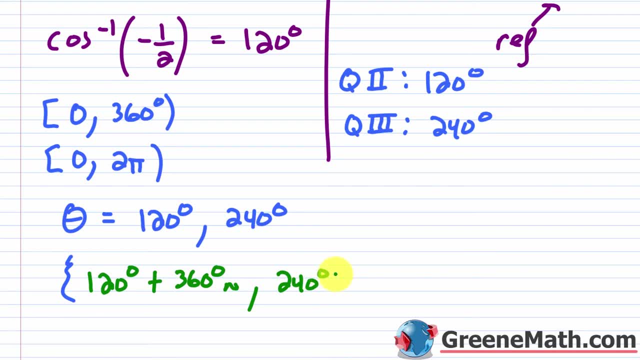 where n is any integer, and then you'd have 240 degrees plus 360 degrees times n, where n is any integer, okay? 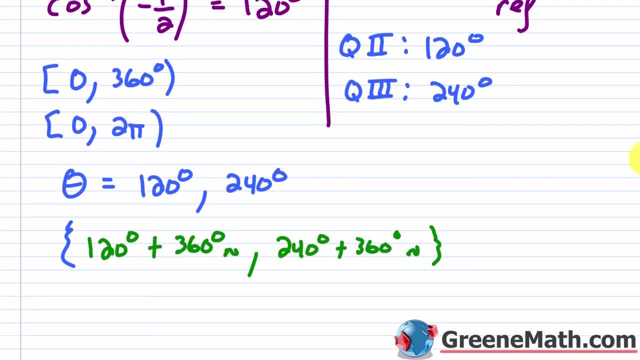 If you want to do this in terms of radians, we can do that as well. No problem. Okay? 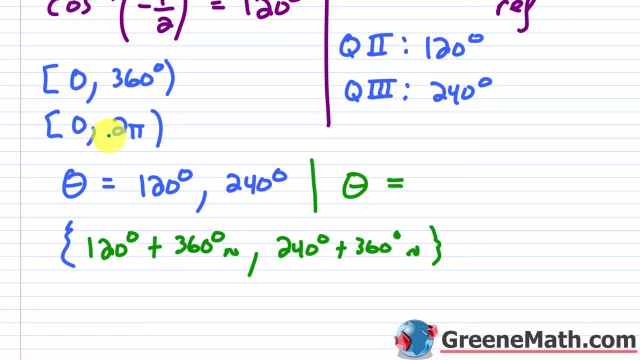 So we would say something like theta is equal to, within this domain, 120 degrees is going to be two pi over three, okay? And then we also have 240 degrees, which is going to be four pi over three, okay? For the general solution, I just go two pi over three plus two pi n, and then I go four pi over three plus two pi n, okay? 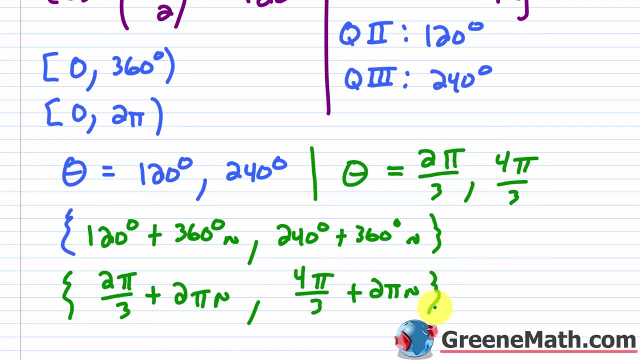 So, again, the period for cosine and sine is 360 degrees or two pi in terms of radians. 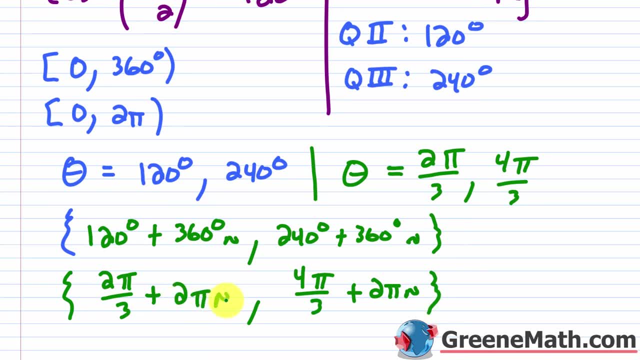 So that's what you want to add. So you have two pi, and then n is just any integer, okay, so that's how you want to do that. 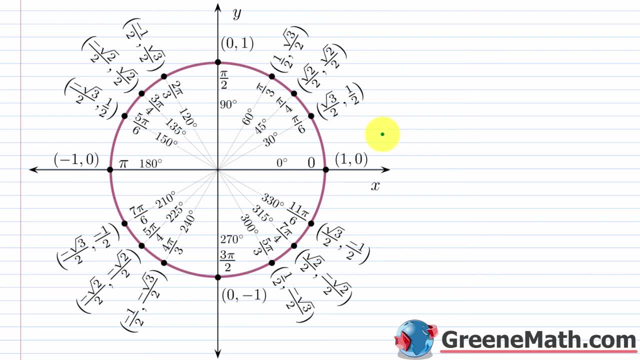 Now, if you wanted to solve this more quickly, especially if it's an easy problem, use the unit circle. So where's the x value negative one half? 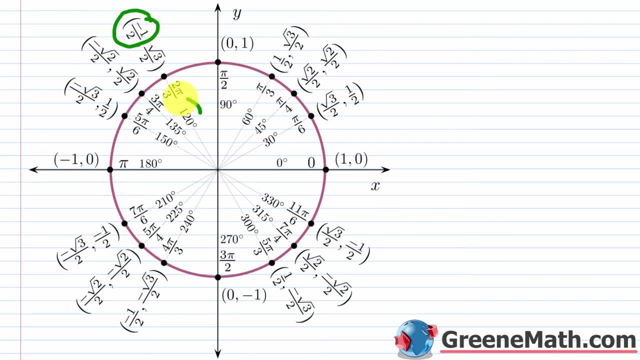 Well, again, you come over here, negative one half is 120 degrees or two pi over three radians, okay? 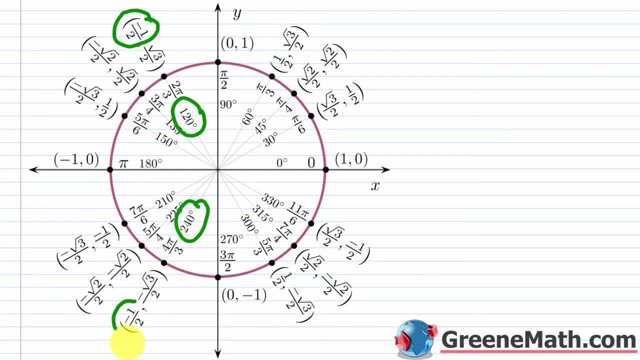 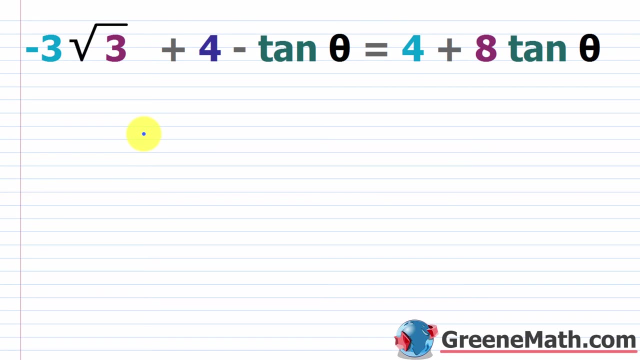 And then also, 240 degrees or four pi over three radians, you got negative one half a square root of three plus four minus tangent of theta is equal to four plus eight times the tangent of theta, okay? So that's what you want to do. So that's what you want to do. Now, let's look at some other problems. Okay, so let's look at one more problem, and this one has tangent involved. Remember, the period for tangent is now going to be pi, okay, or 180 degrees. So you have to keep that in mind here. 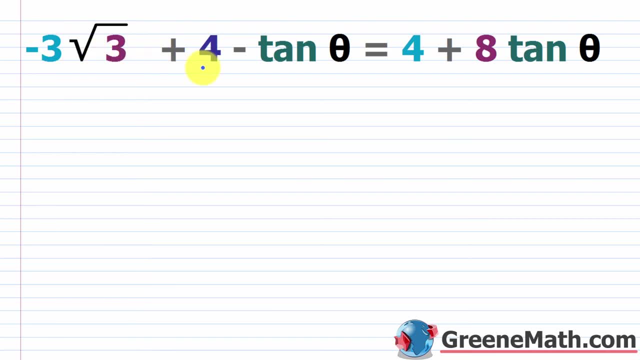 So if I have something like the negative of the square root of three plus four minus tangent of theta is equal to four plus eight times the tangent of theta. Okay? Well, immediately, I can just get rid of the four from each side, right? Same thing on each side, just get rid of it. 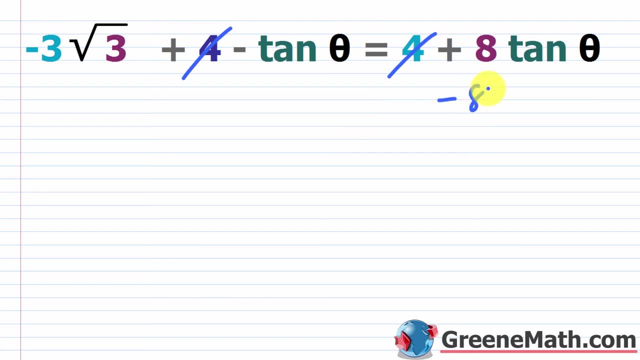 And what I want to do now, let me go ahead and subtract eight times the tangent of theta away from each side of this guy. So I forgot my eight. So minus eight times the tangent of theta, okay? So this will cancel out over here, okay? And I'm just going to add three times the square root of three to both sides. So what I'm going to end up with is you can put a negative one there. You'll say you have negative nine times the tangent of theta is equal to three times square root of three. Divide both sides by negative nine, okay? 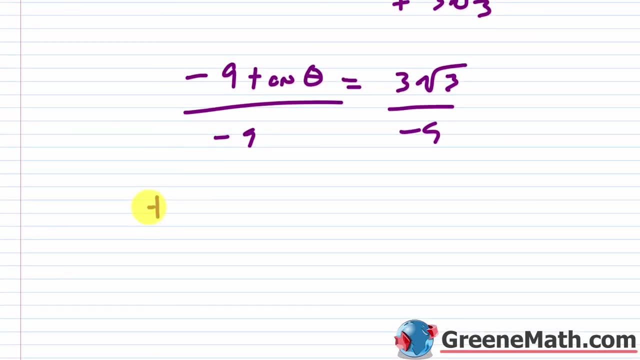 Let me scroll down just a little bit, and I'll say that I have the tangent of theta is equal to the three is going to cancel with the nine. This is a one. This is a three. So let's say the negative of the square root of three over three. Okay. 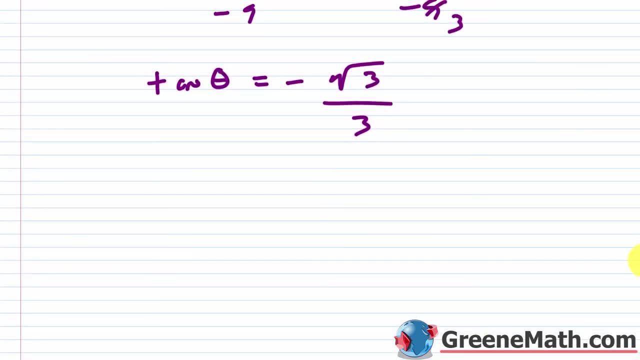 So now with tangent, it is a little bit more challenging to think about these. You could use your special triangles in this particular case, and just think about the square root of three over three. 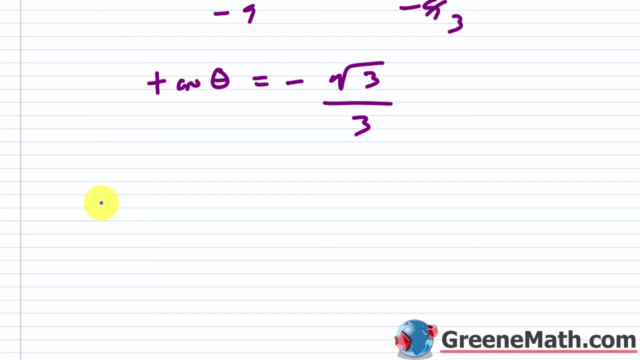 The tangent of 30 degrees is square root of three over three. So let me just write this over here. The tangent of 30 degrees is equal to the square root of three over three. 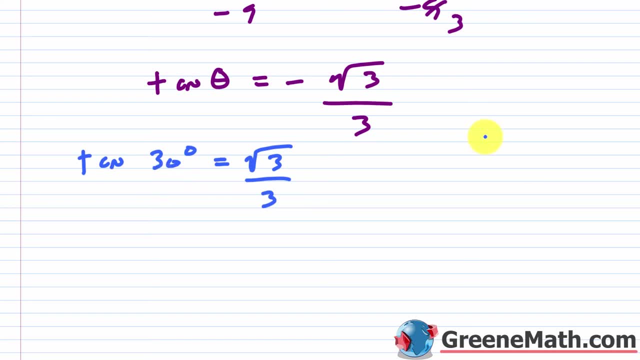 So again, I would say that tangent is going to be negative where? Let me draw this out here so we remember this. So we remember the all students take calculus. So tangent is negative in quadrants four and two, okay? 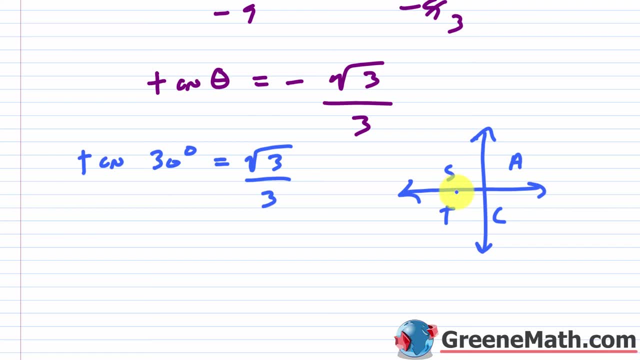 So let's think about this. In quadrant two, where would I have a 30 degree reference angle? Again, if I take 180 degrees and I subtract off 30 degrees, that gives me 150 degrees. 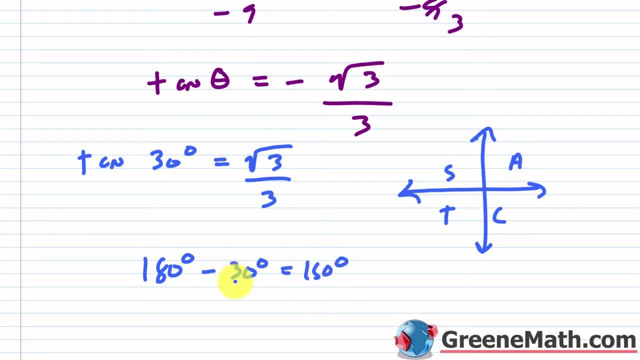 Okay. My reference angle here for 150 degree angle would be 30 degrees. 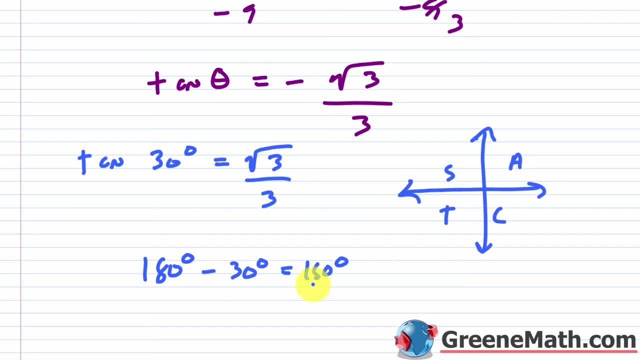 So my value here, if I did tangent of 150 degrees, because it's negative, I would get the negative square root of three over three. Okay. 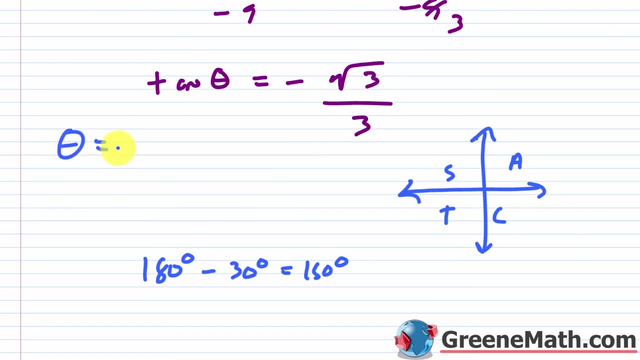 So let me erase this for a second. Let me just put one answer here. So theta here would be 150 degrees. Okay. So this is 150 degrees. 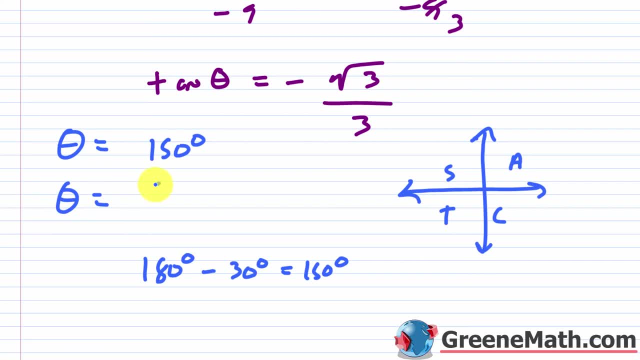 Or again, if you want to write this in terms of radians, this is five pi over six. Okay. Whatever you want to do. 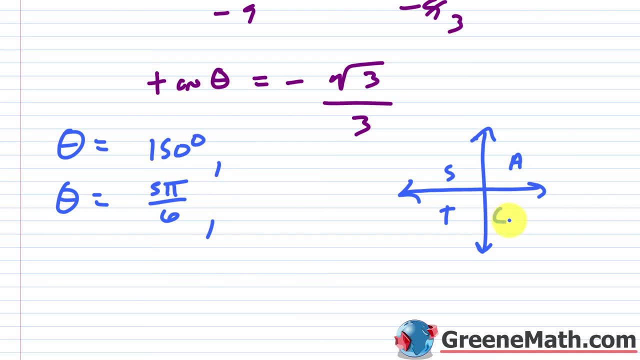 So let me erase this for a second. Let's think about in quadrant four. So remember I said the period when you work with tangent is 180 degrees. 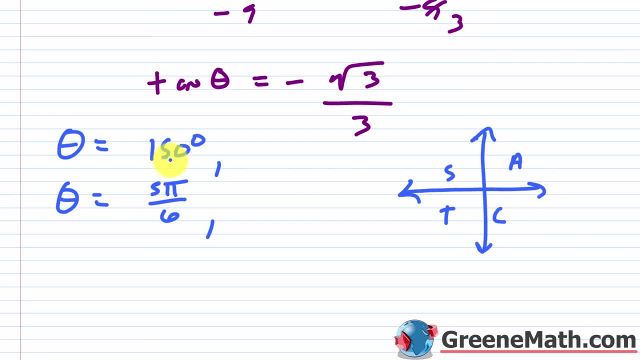 So I can just add 180 degrees to this. Okay. 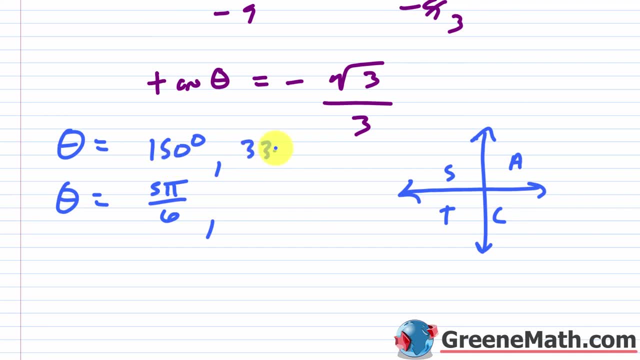 So 150 degrees plus 180 degrees is going to be 330 degrees. Okay. 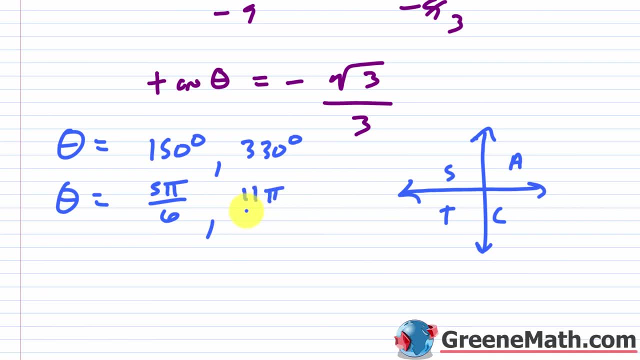 Also, what you could have done, and this is 11 pi over six in terms of radians. Also, what you could have done is, again, look for a 30 degree reference angle in quadrant four. So in quadrant four, I would just go 360 degrees minus 30 degrees is going to give me 330 degrees. So this is the angle I'm looking for. All right. So obviously these would be your solutions if you had a domain restriction. Okay. 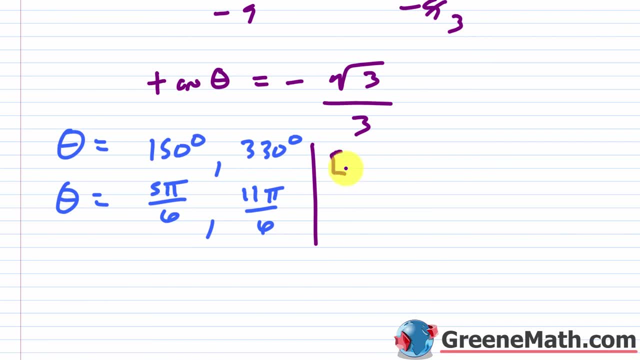 But if you didn't have a domain restriction, let me just write this over here. So this is zero to 360 degrees. And this one is zero to two pi. Okay. In terms of radians. If you didn't have a domain restriction, you have to be careful because a lot of students will come through here.